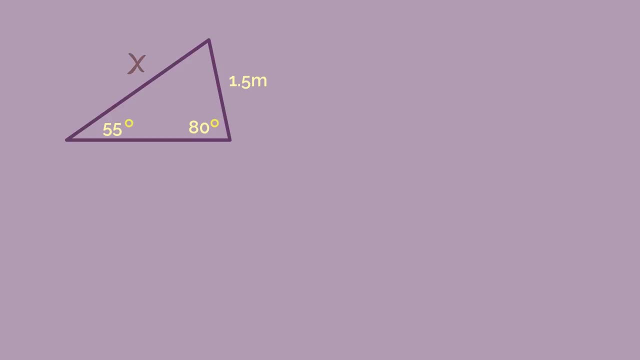 So start by labelling the sides as A and B And the angles as capital A and capital B. So let's call 1.5cm side A, 55 degrees must be angle A, And so then 80 degrees is angle B. 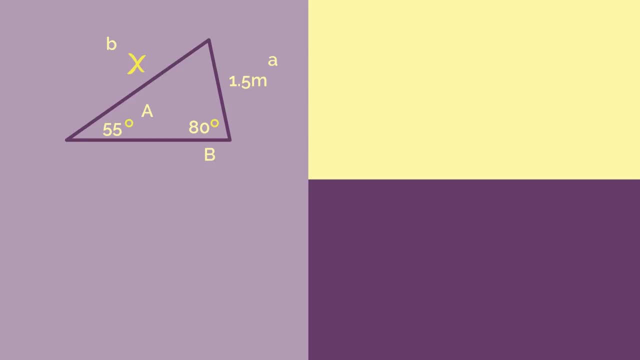 Which means the missing side x is little b. We need to find a missing side, So we'll use this version of the formula. So we just substitute in the numbers And we get: 1.5 divided by sine 55 equals b divided by sine 80.. 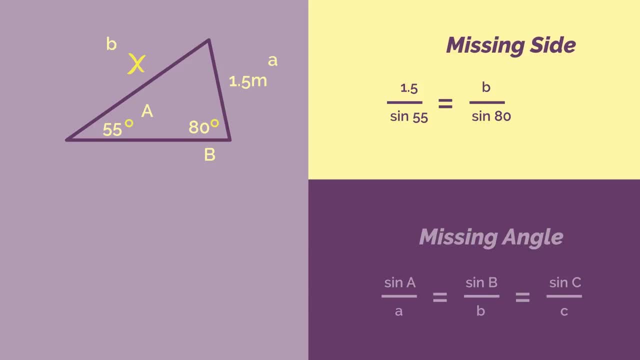 So to get b on its own, we do some simple rearranging By multiplying both sides by sine 80.. And then these ones cancel each other out And we're left with b equals 1.5 divided by sine 55, multiplied by sine 80. 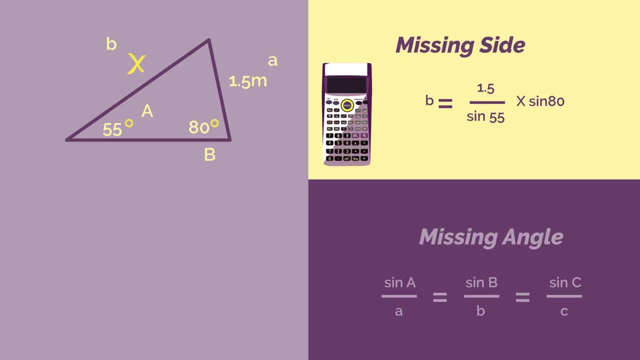 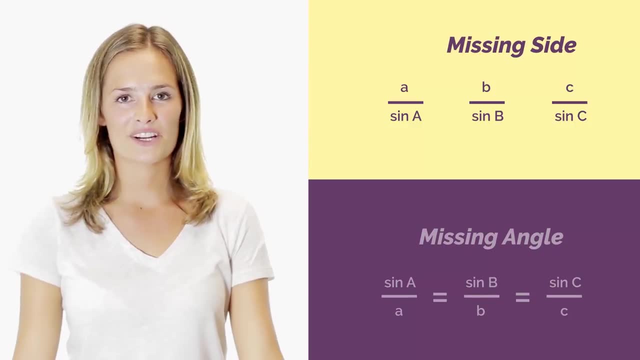 Which we can enter into our calculator, And this gives us 1.8m. So let's now have a look at an example where we're trying to find a missing angle. So we need to use this version of the sine rule: The missing angle version. 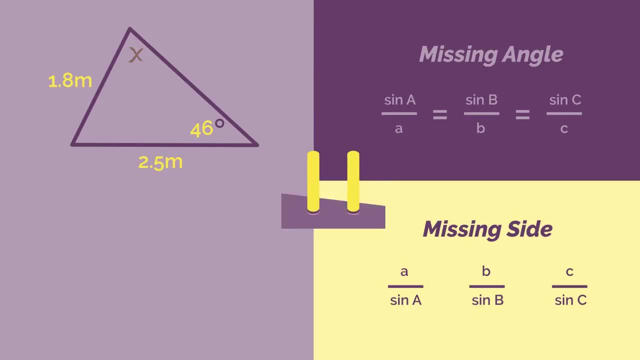 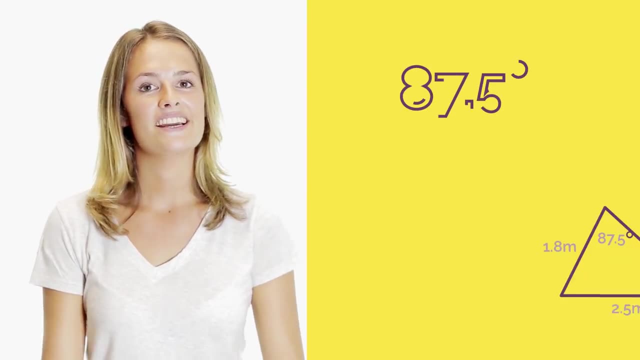 Give this one a go yourself. Pause the video, Work out the answer And click play when you're ready to check. Did you get 87.5 degrees? If you did and you want to skip the explanation, Click here. Otherwise, let's go through it together. 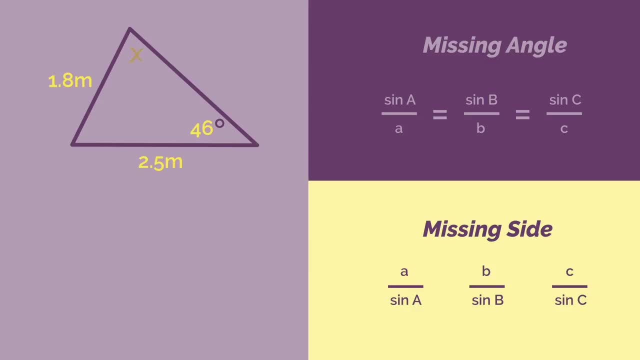 So we start by labelling the sides and angles with a's and b's. So I'm going to label 1.8m as a, So therefore 46 degrees must be angle a. So then 2.5 is side b. 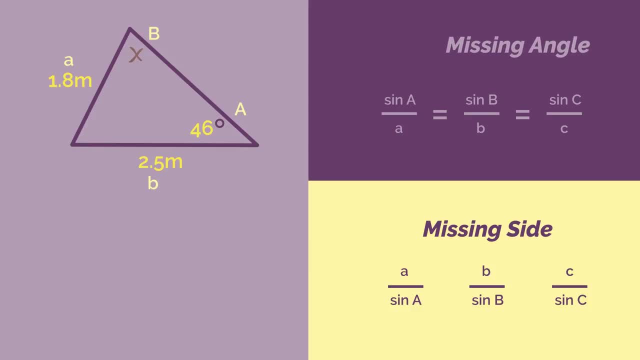 And the missing angle x is capital b. Again, just substitute the numbers into the formula And we get sine 46 divided by 1.8 equals sine x divided by 2.5.. A little bit of rearranging. So multiply both sides by 2.5. 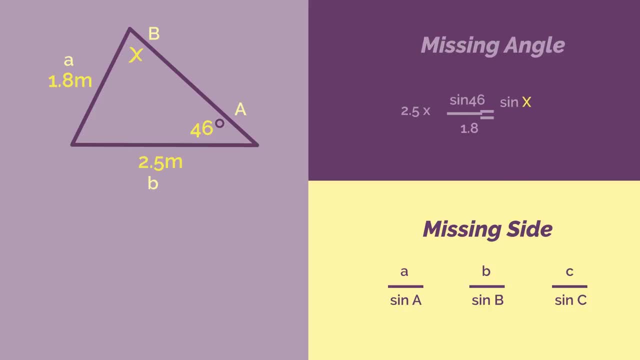 And they cancel out on this side, And we get 2.5 multiplied by sine, 46 divided by 1.8. Which we can enter into our calculator. So then sine x equals 0.999, and so on. Remember, to get x on its own we must use inverse sine.